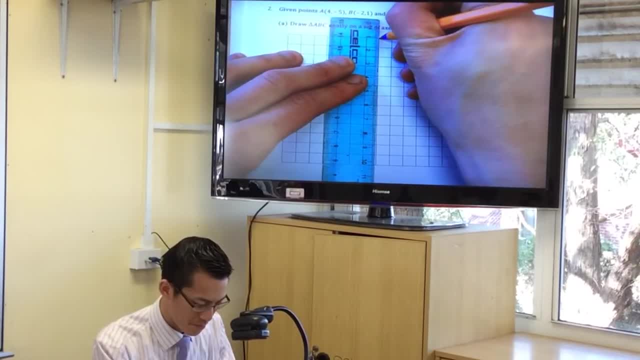 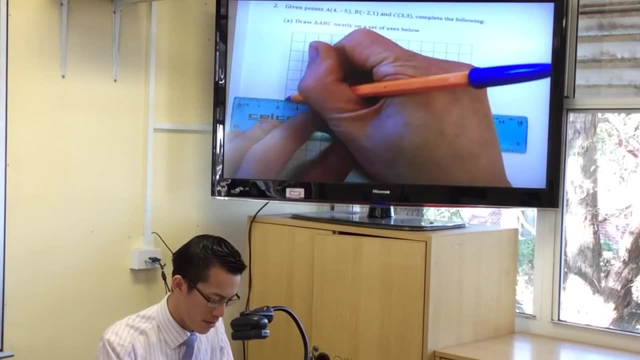 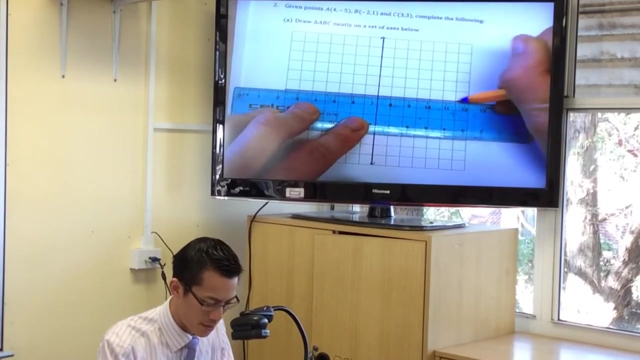 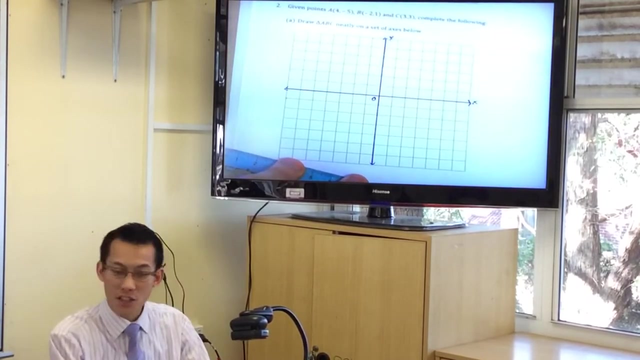 the middle. okay, Like this: That looks pretty close to the middle, right, Yeah, that's acceptable. Negative five: There isn't a middle for this one, I don't think, But that's close enough. Okay, so you've got your zero, your y-axis, your x-axis, So again, I'm going to do this in order. 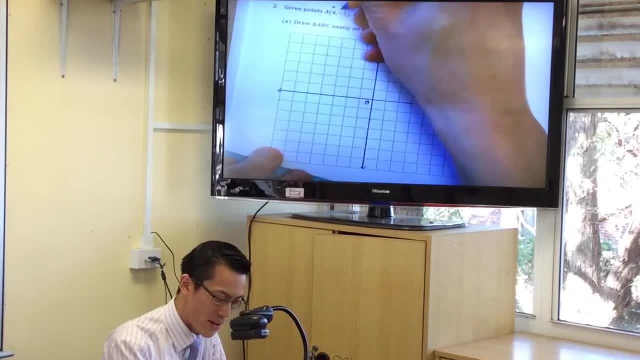 Four negative five. Again, I'm going to do this in order, Okay. so you've got your zero, your y-axis, your x-axis, So again, I'm going to do this in order. Again, that's my x-value, my y-value, okay, So when x is four, that means go across one, two, three, four. 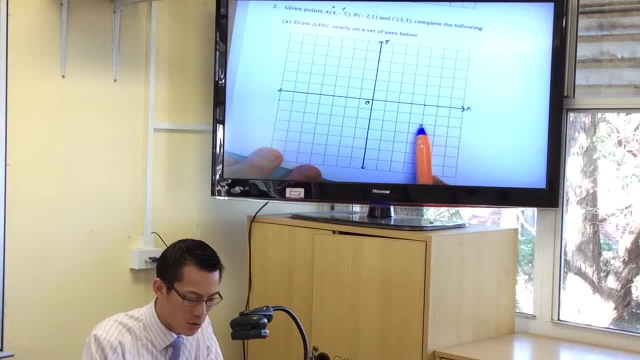 And y equals negative. five means go down one, two, three, four, five. There he is right there. Can you see it? Okay, it's a good idea. It's a good idea Because then you can tell the points apart, you don't get confused. 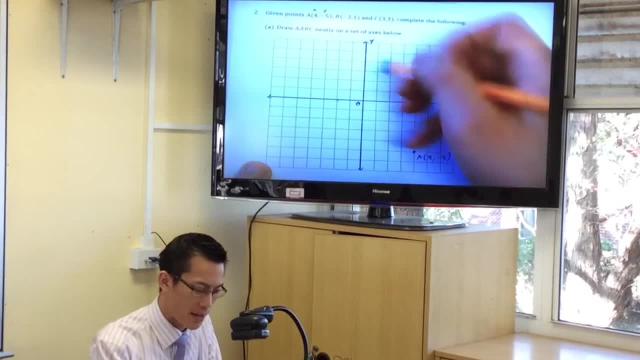 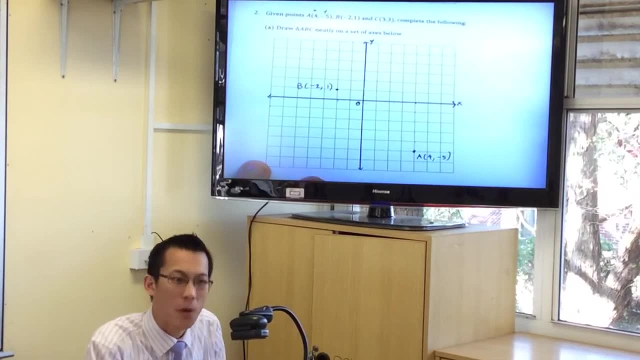 B is negative. two, that's negative. one. two, I'm going to the left, and one. So there you go. And last one: three, three. I think it's a good idea. where you can Like sometimes if you've got lots and lots of points flying around, maybe you want to avoid putting on so much information. 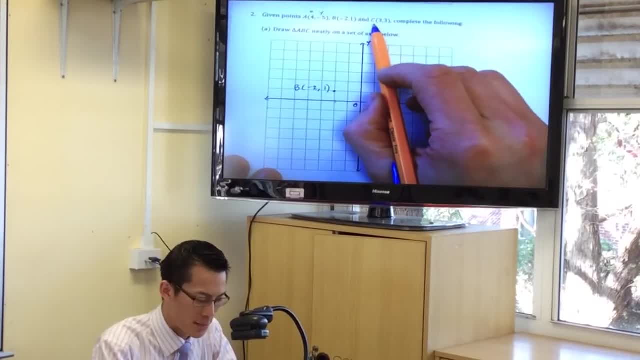 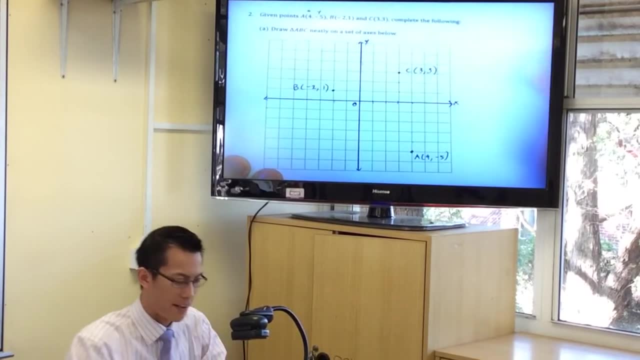 But I'm just going to draw a triangle in a second. It's pretty simple. Last point: three, three. So one, two, three, One, two, three. There you go. There's C. Okay, now you'll know if you got it right or not by the last step, which is it says: don't just plot the points. 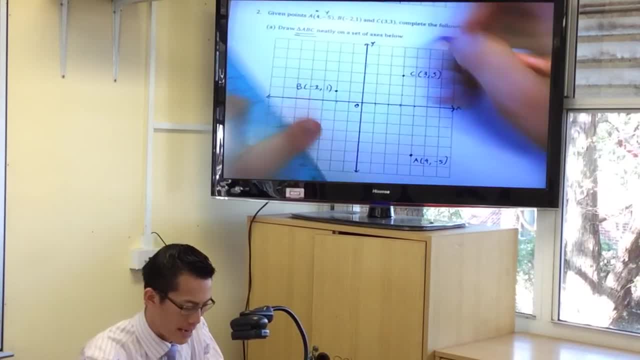 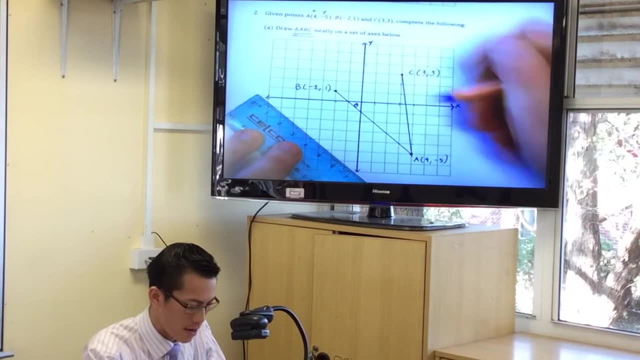 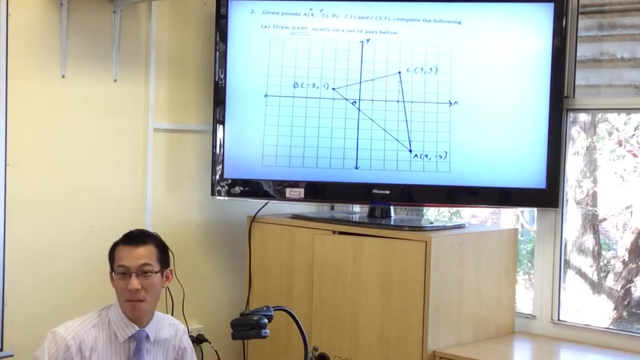 It says: draw the triangle. Okay, so I'm going to join these guys up like so There's a C, there's a B and there's a B C. There you go. So you're trying to look something like that. 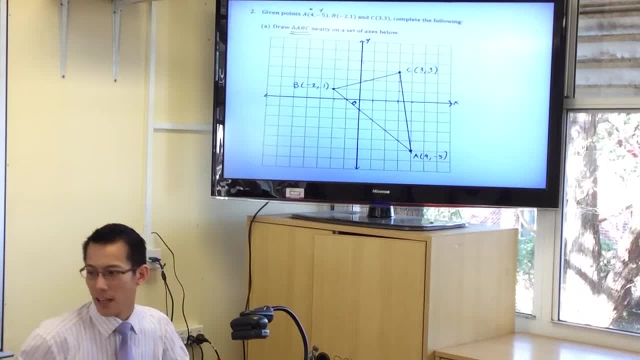 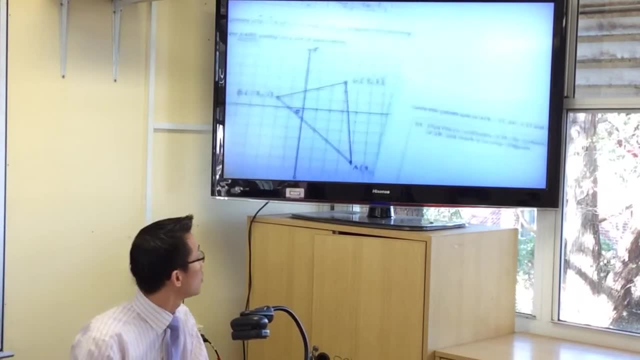 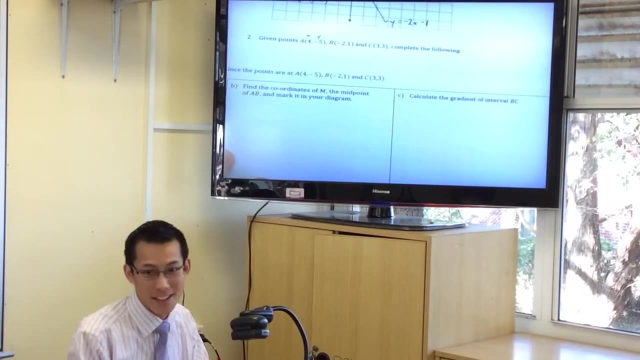 Okay, Now there's something a bit sneaky. I'll just get this piece of paper here because I've got two. The next page, right. If you have a look, It starts talking about all these other things, but you might notice the three coordinates they give you. it's the same coordinates, right? 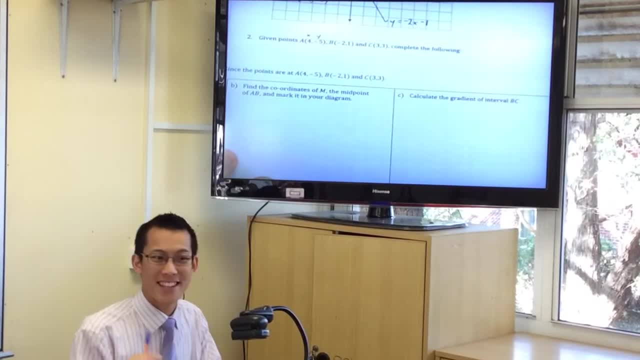 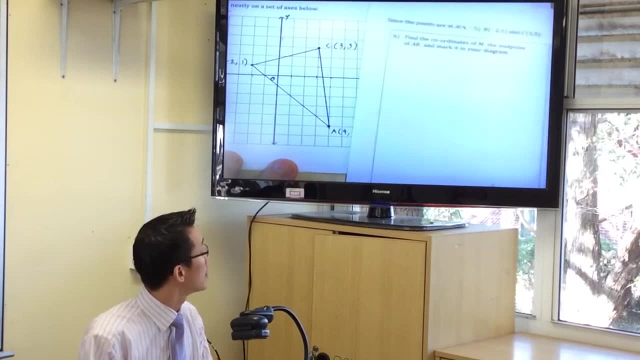 So you can actually use the diagram you did before to help you out. Okay, so here's what I'm going to do. I'm just going to have this diagram here, just off on the side, while I refer to these questions here. 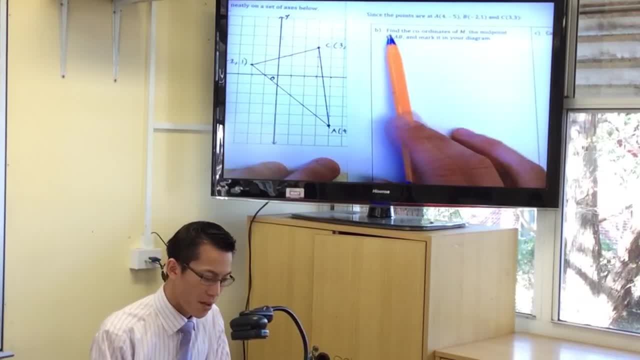 Okay, So find the, it is the same. How do you think Find? in fact, it says you know, since the point R, right, Like it's talking about, and this is part B, following on from part A. 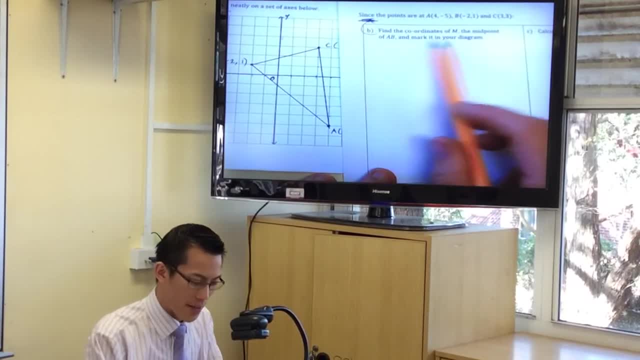 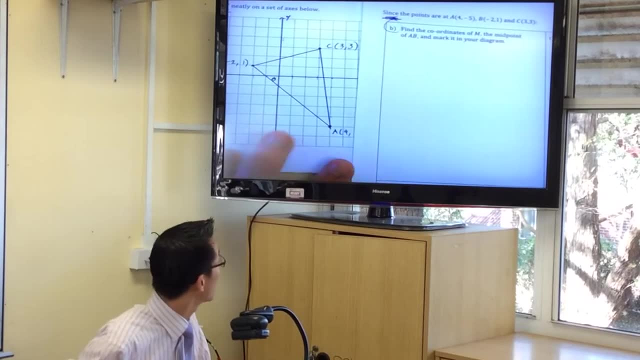 So it's all one One question: Find the coordinates of M, the midpoint of AB, and mark it in on your diagram. Okay, Now we're going to do this precisely, but in a second, before we do that, you have a look at this line AB. 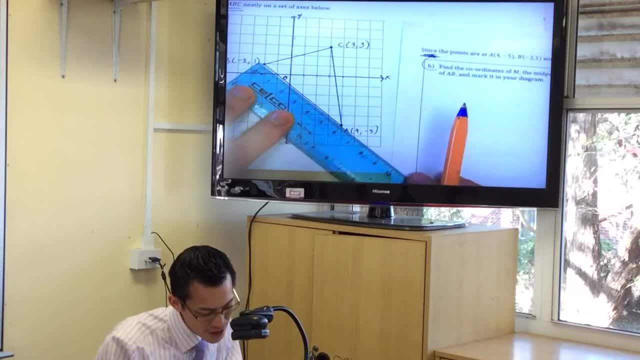 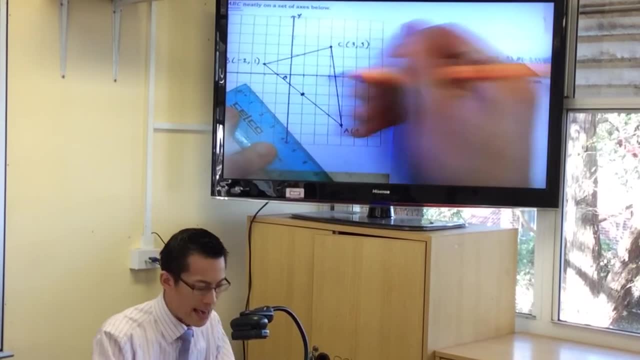 You can. actually, if you had a ruler, you could get it out And you could say: well, it looks like it's about six enemies long, right, I think it's going to be here. I expect it to be there. 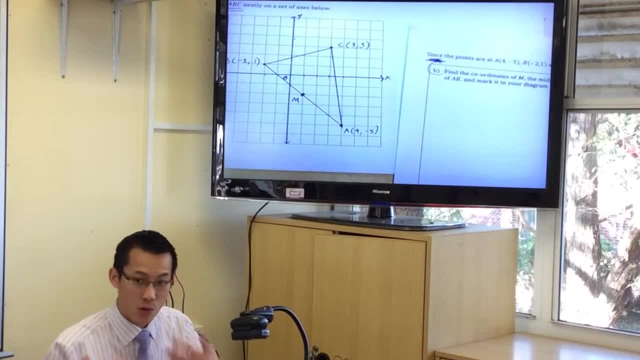 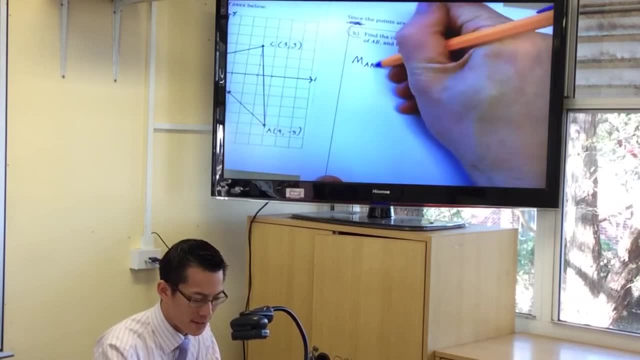 Okay, Now, that's just roughly approximating it. Let's crunch the numbers and see if it works. It works out, Okay. So here's what I've got. What is the midpoint formula? Does anyone remember? Yes, I'll give you a clue. 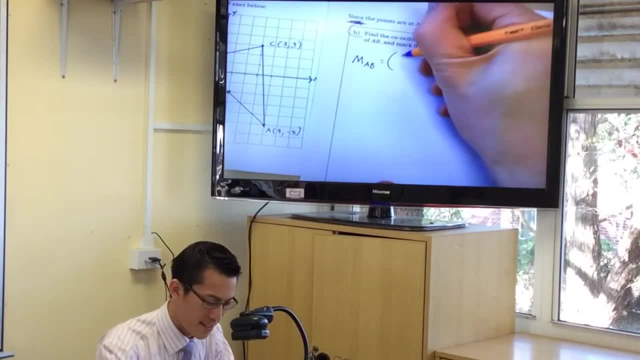 It starts with these big brackets: Bracket X1.. Yes, X1.. Y1. Whoa, whoa, whoa. Before I do my X1,, before I go to my Ys plus X2.. This is the midpoint. 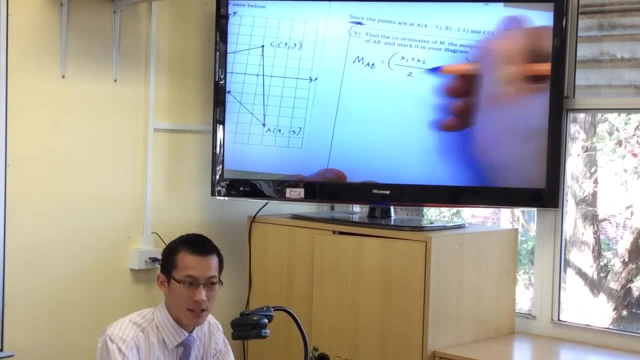 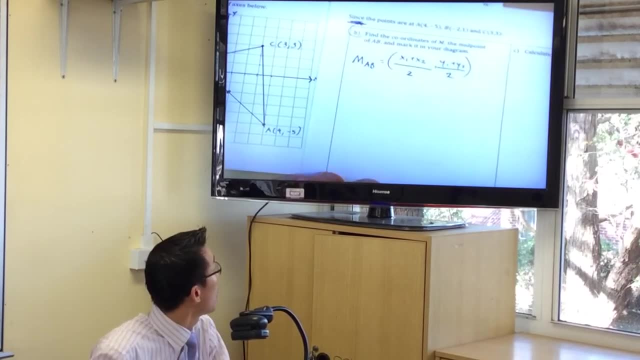 This is the most recent one we learned. And then I divide by two, because I'm taking the average, And then you do the same thing for the Ys, Like so, Yes, Okay, So I've got my Xs and Ys. 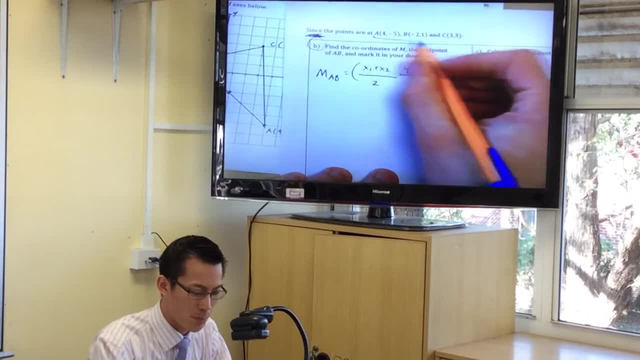 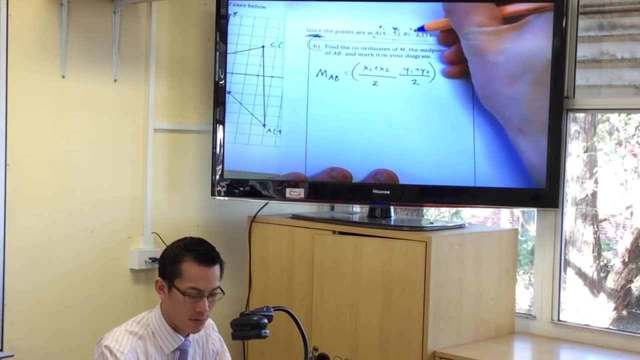 Now I'm going to label them up here. These are the two points I'm interested in, So I'll call that X1- Y1 and X2- Y2, like so Okay, So now all I need to do is process it with these particular values. 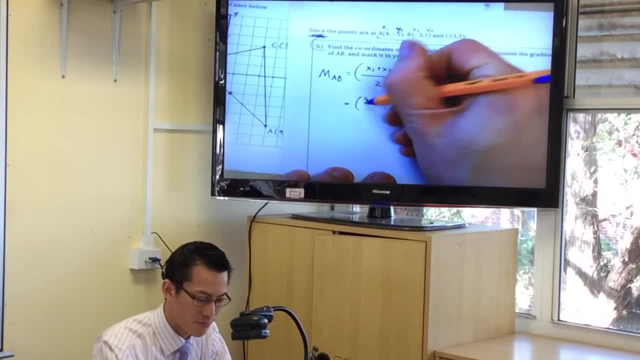 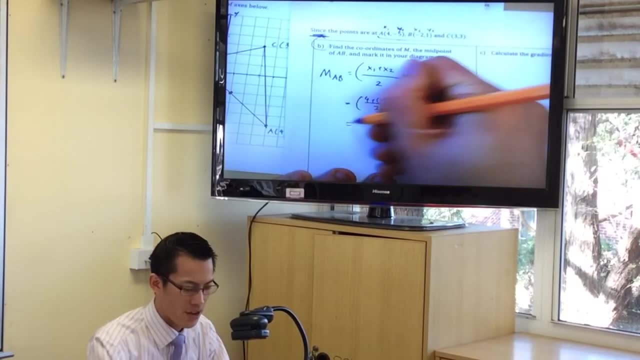 So I get 4 plus negative 2 and negative 5 plus 1.. Okay, You guys can help me out. 4 plus negative 2, what's that? 2 over 2.. That's 2 over 2, good, which is 1, right. 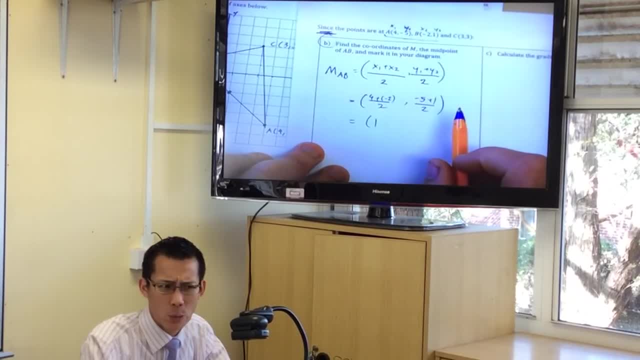 And then it's minus 4.. Minus 5 plus 1.. What's minus 5 plus 1?? Minus 4. That's minus 4.. You divide by 2.. Oh no, I did it right. 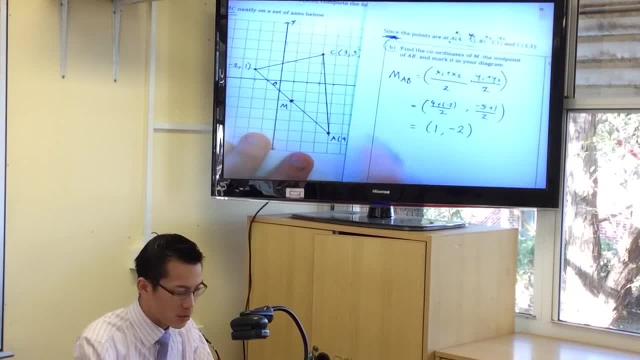 Gives you negative 2.. Now does that check out. You have a look. I did it right. That looks right. Look see: 1 across and 2 down. Sure enough, it's 1, negative 2.. 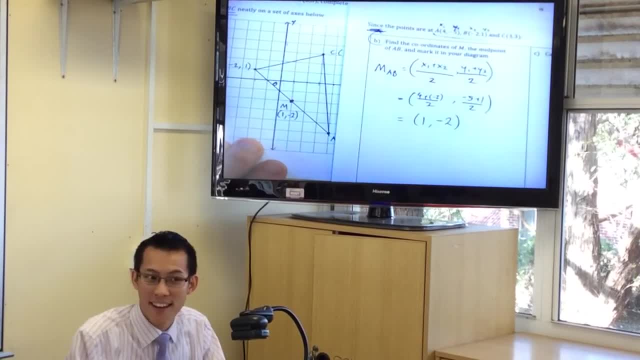 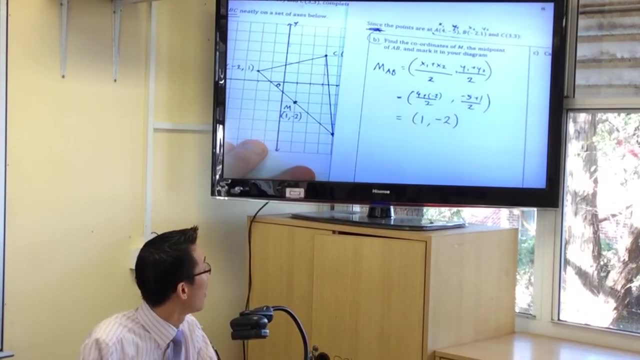 I did it. I did it So good. Okay, Well done. Any questions on that? Does anyone want me to clarify any steps? Just just Okay, I'll try to move over. I'm scared, I'm fucking my nails. 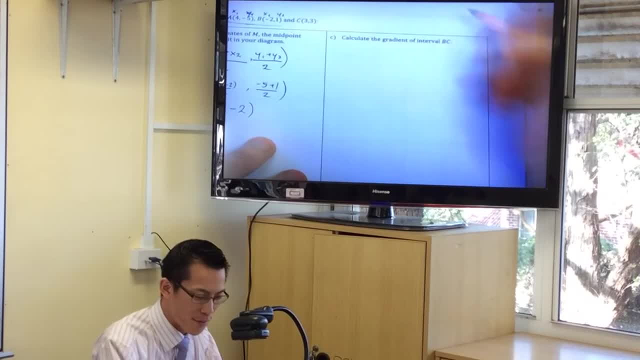 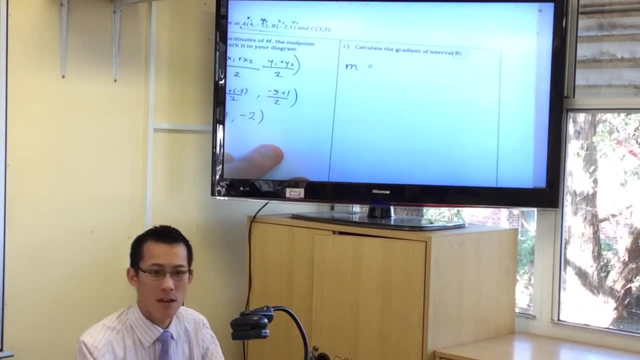 Yeah, you are Okay. Calculate the gradient of BC. Okay, So I need the gradient. that's a lowercase m, right? What's the gradient formula? Rise over run, Rise over run. very good Ding, That's excellent. 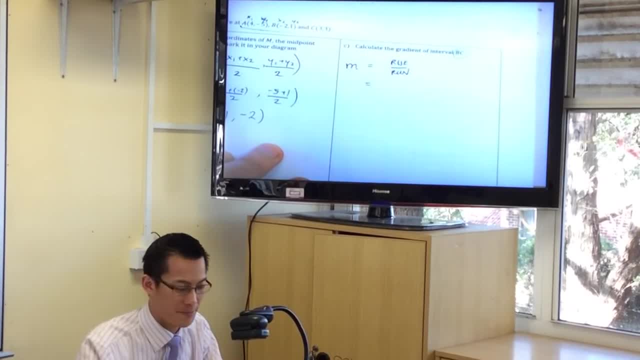 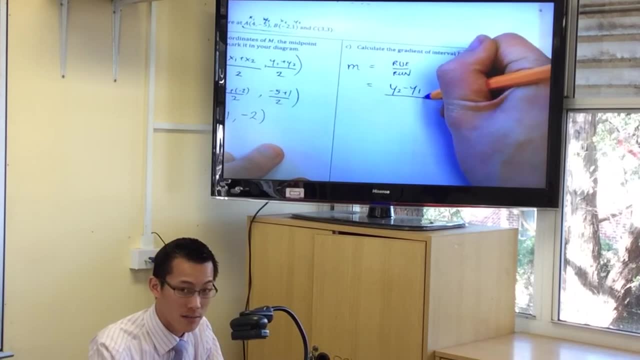 Now what are the x's and y's that correspond to that? x1, y1.. Rise is about the y values, right, So I'm going to have y2 minus y1 over, And then what? And then run is about the x values. yeah. 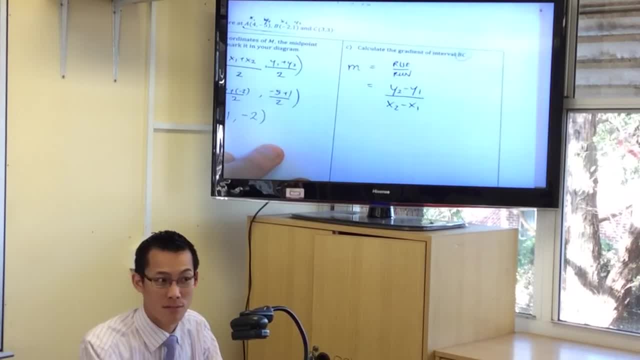 x2 minus x1, yeah, Yes, Okay. So let's have a look. Here are my points, right? I'll just write them over here, just so I can see them right next to each other. right, There you go. 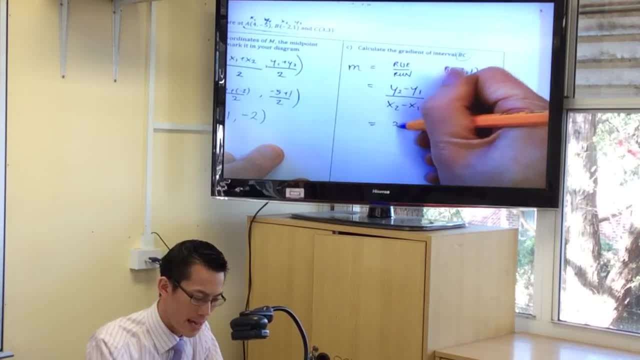 So y2 minus y1, I'm going to go 3 minus 1,, like so, And then run is 3 minus. now watch out for the double negative. like so, 3 minus 1 is 2.. What's the denominator? 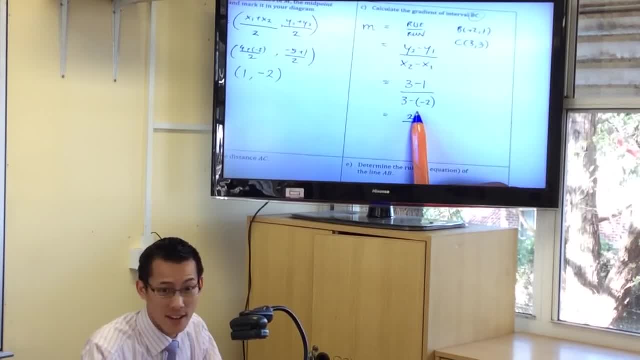 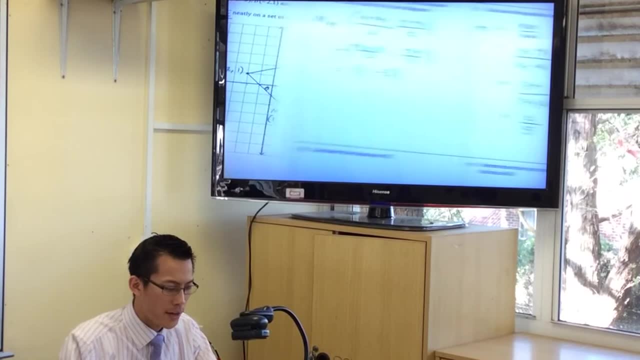 3 minus negative 2, what's that? I think that's 5, isn't it? Yes, Double negative equals a positive. Now just check that out. 2 fifths- Does that look about right? Yeah, look see. 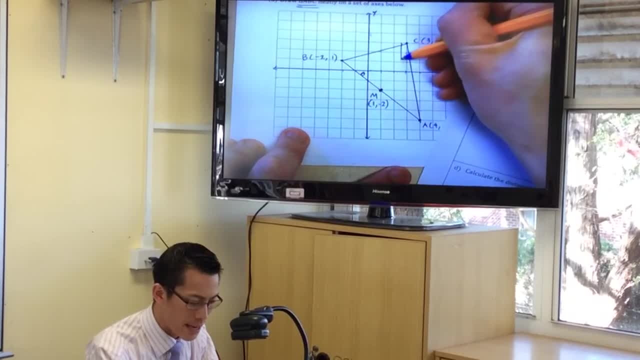 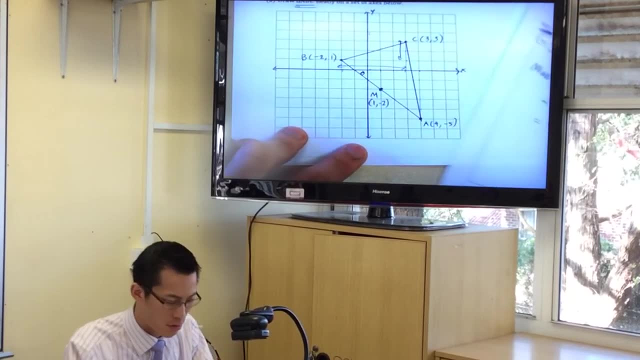 It goes the rise. the rise here is 2 units and the run, like that, is 5 units. right, Rise over run 2 over 5.. Awesome, Okay, We're almost there. Okay, Calculate the distance AC. 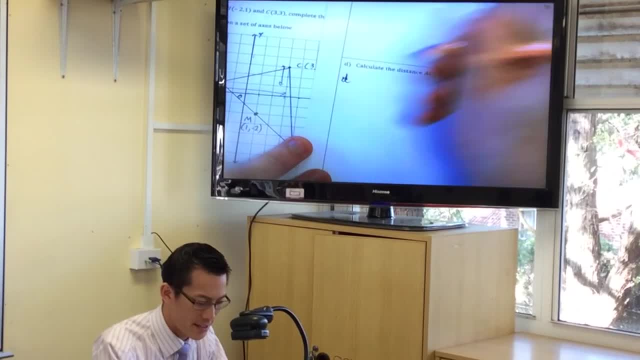 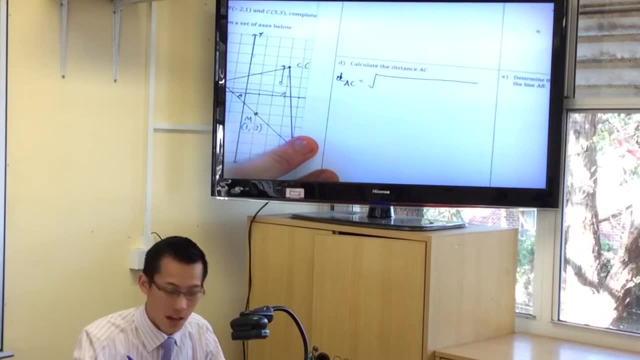 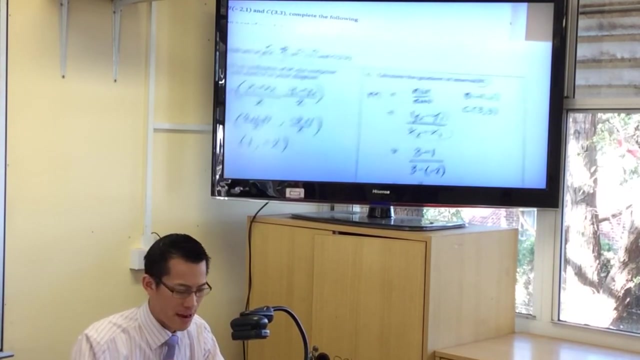 Alright, this is the long, awkward formula: Distance AC. I'll give you a clue. It's got that square root sign. What's underneath the square root? Yeah, yeah, It's the same as these guys, right? Except they're because from Pythagoras they're squared right. 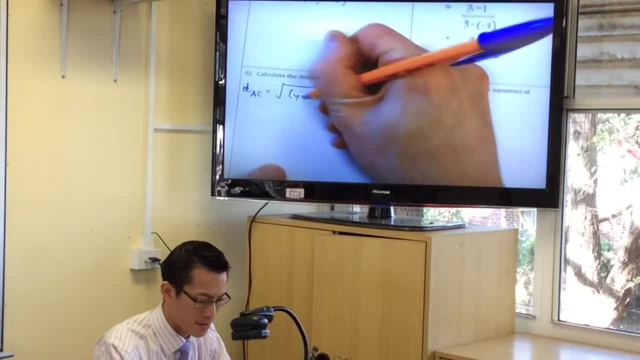 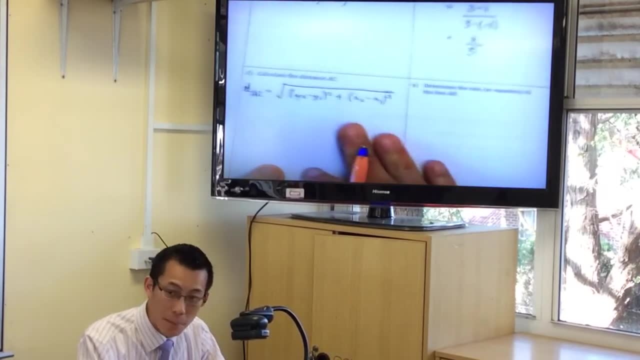 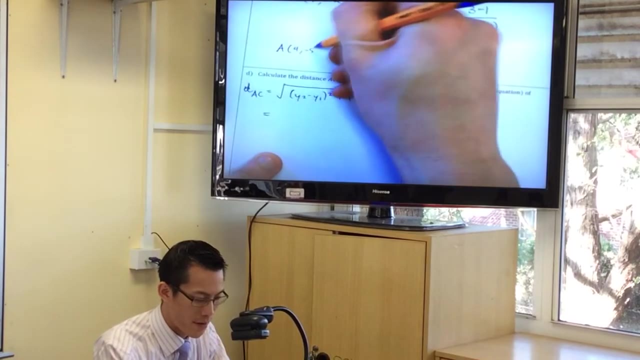 So I'm going to write it like this Squared And the x's Squared. Okay, So this comes from Pythagoras, right? So now I look at my numbers. I've got my. my A is 4 negative 5 and my C is 3, 3.. 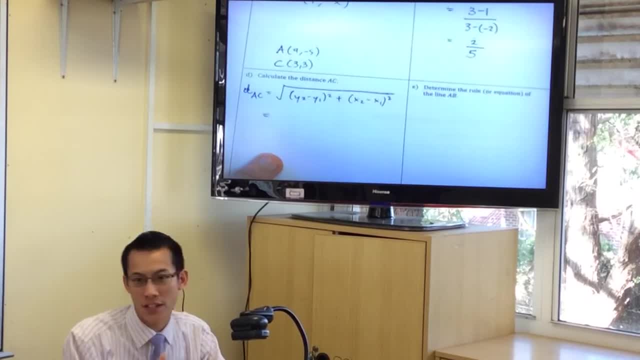 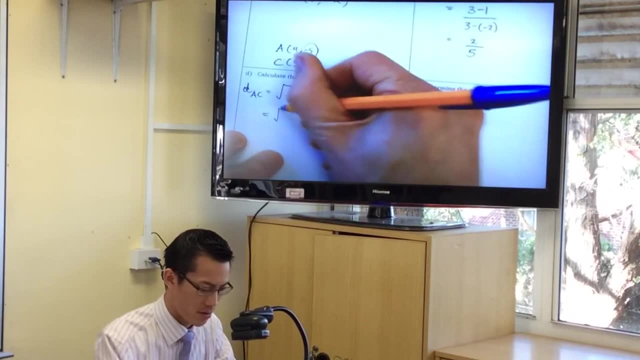 You can see, I keep on writing the coordinates every time, so I know which ones I'm referring to and I don't mix them up. It's really easy to mix them up. Okay, Here's the y values. So square root of 3 minus negative 5.. 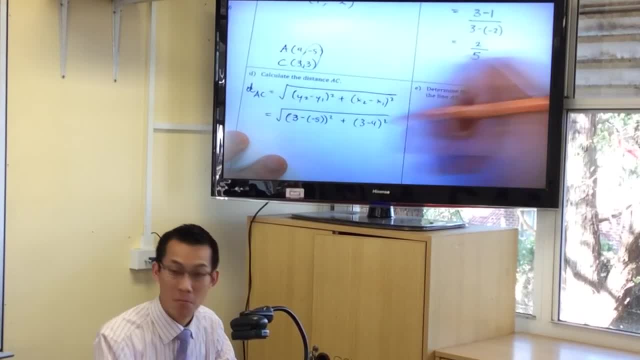 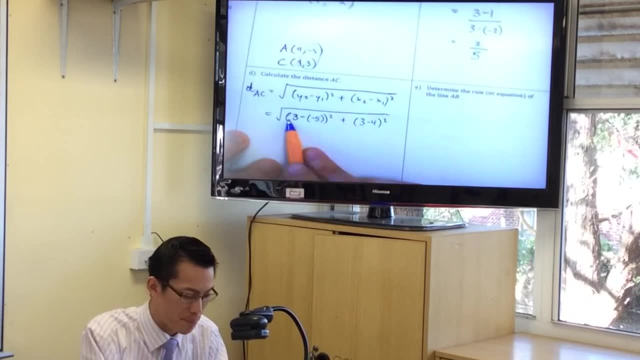 3 minus negative, 5.. And then this one will be 3 minus 4.. What's 3 minus negative 5?? 3 minus negative. It's a double negative. So it'll be 3 plus 5, which is 8.. 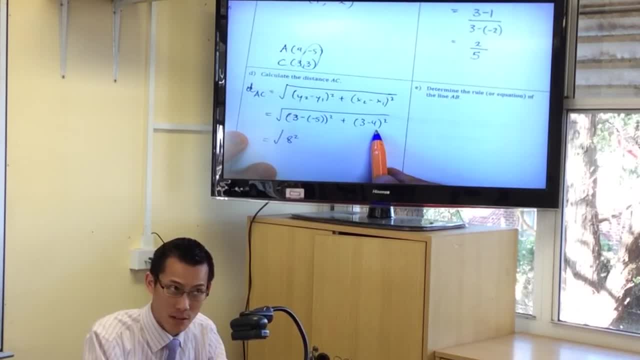 Well done. 8 squared, 3 minus 4 is negative 1.. So when you square it, what happens? Negative 1 times negative 1. The negatives cancel each other. Yeah, So it's just going to become 1.. 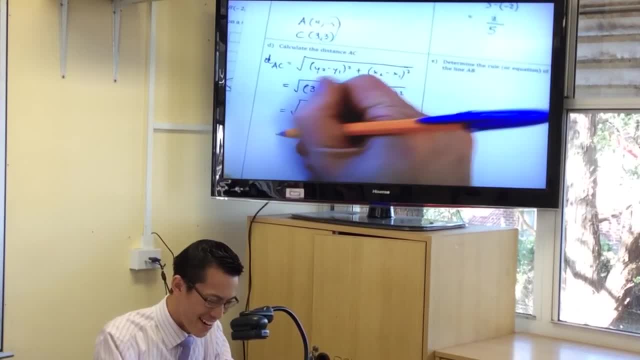 There's a song about it. There's a song about it. I was like, okay, Just one, All right. So then, almost finished, 8 times 8.. 8 squared, What's that? equal to 64.. 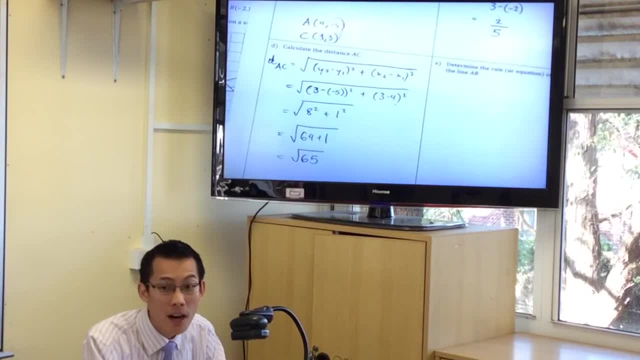 64.. Very good, Plus 1.. 64 plus 1 is 65.. Is 65 a squared number? No, No, No, it's not. Did they ask you to approximate? No, No, So you just, you just say units. 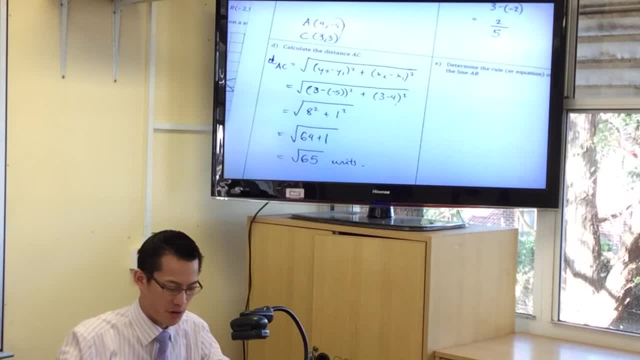 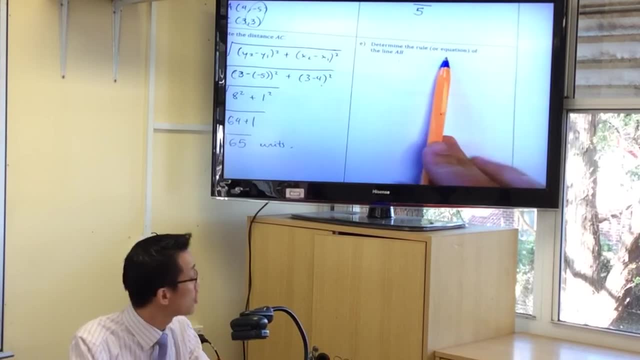 Done, Okay, Which would be like 8.1 or something I don't know, 8.2.. Something like that, But that's, that's finished. Yeah, Okay. Next step: Determine the rule or equation of the line AB. 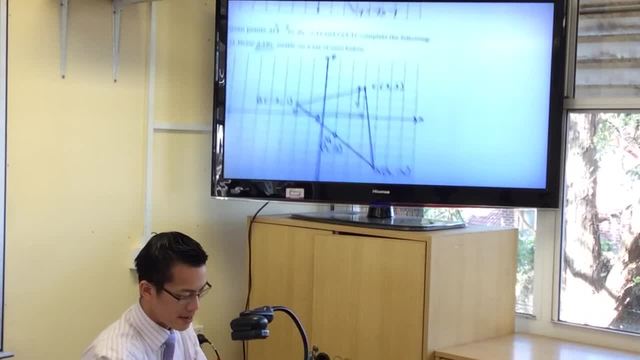 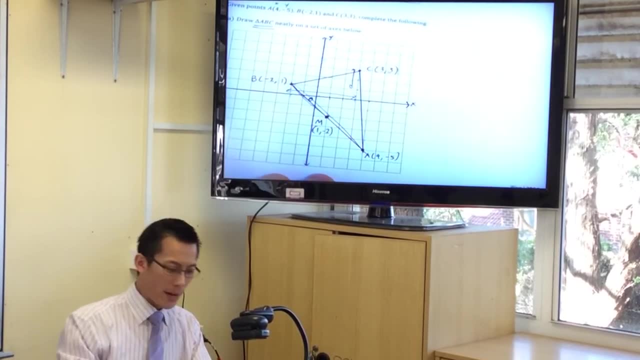 Now let me just put it on the picture again: AB, That's, that's this line here, Right, What? This line here? Okay, So how are we going to do it? What are we going to do? This is, this is my many, many lines. 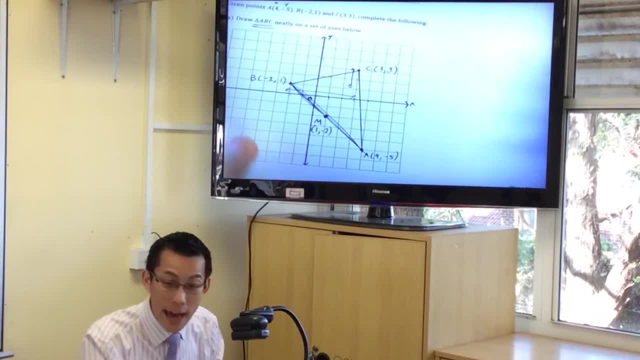 Okay, We need two pieces. We need two pieces. I need a y-intercept- That's, that's this one here- And I need a gradient: A y-intercept and a gradient. So can you read off Like I've done it. 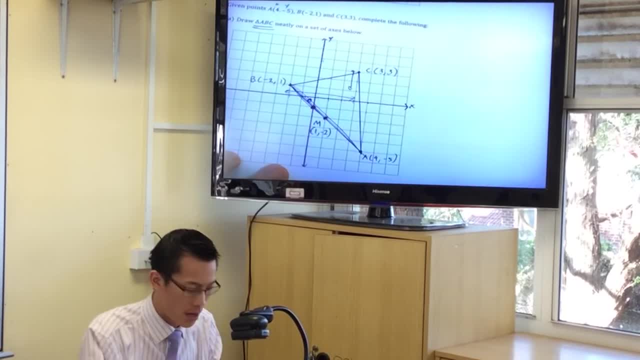 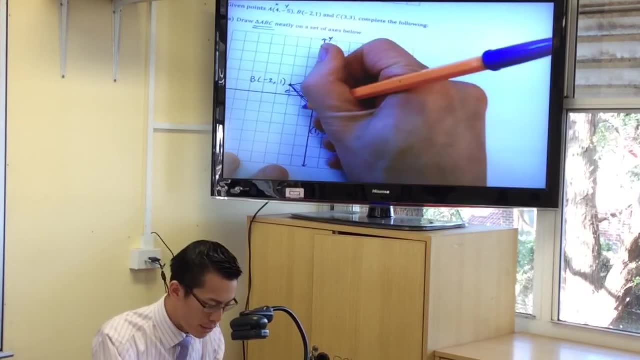 One grid square is one unit. Yeah, So what we're going to do is we're going to do a gradient. Okay, What would that value be? It's just one below the origin. Yeah, So it should be negative one. 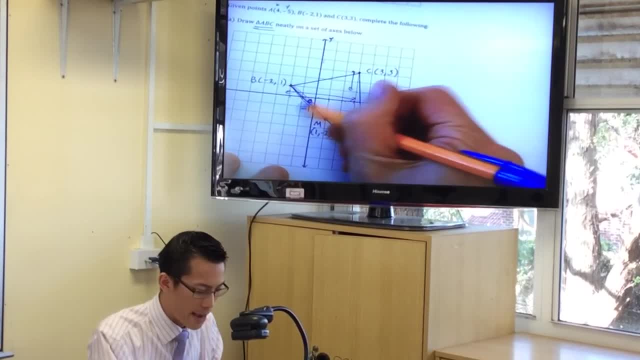 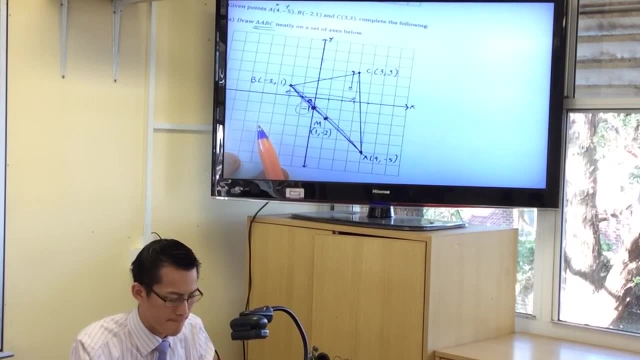 One, One, Very good, Okay, So that's my y-intercept. I'll just tuck that away. Okay, Now, what's the gradient? This is a bit trickier. What's the gradient Two, Four: